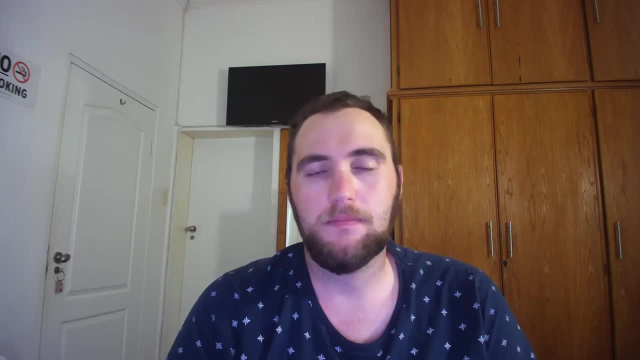 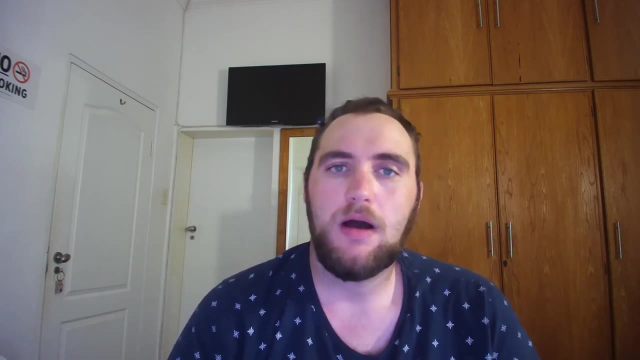 they're the most popular web browsers out there. i didn't include microsoft edge because it was very difficult to get the out of the box experience for me on my computer, so i avoided that one and i chose the brave browser, because it's a new browser i found recently that is really good at. 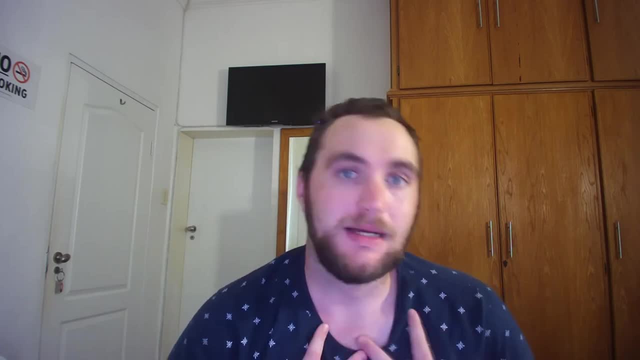 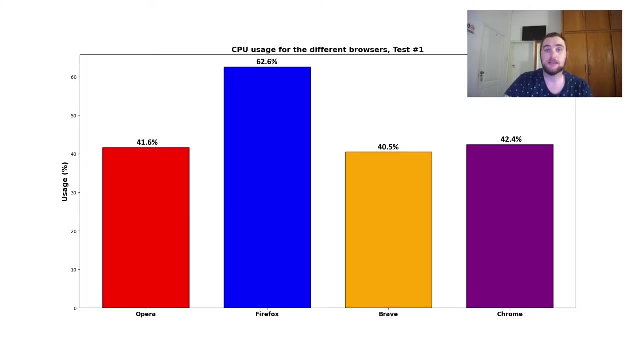 the whole privacy thing. so i just also wanted to see for myself in general how it performs amongst these other web browsers out there. so the very first test result i want to look at is the cpu usage for just one video playing. nothing else is running in the background. 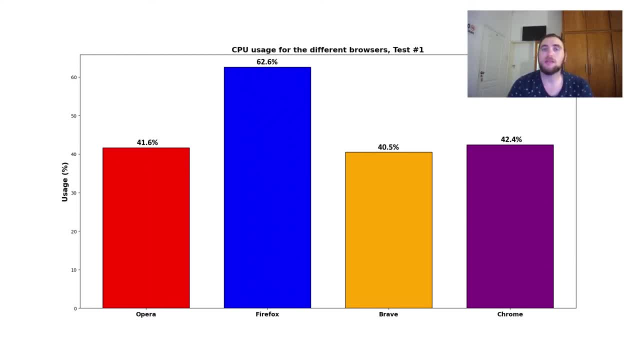 and from this test you can see that the web browser that is performing the best is the brave browser, using 40.5 of my cpu, but in terms of the worst performance it's mozilla firefox, using 62.6 of my cpu usage. now, this is a very artificial result because in reality, when i was watching, 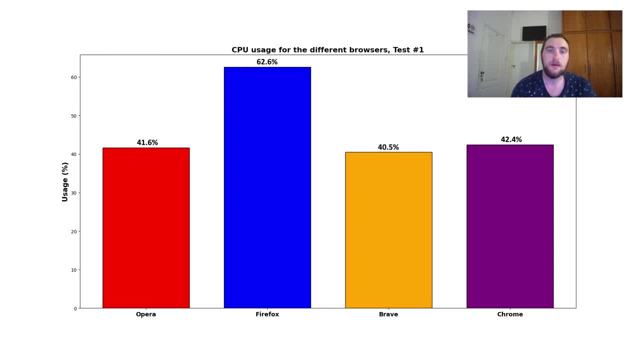 the video. i was also moving the mouse cursor around a lot on the video. if i just put the mouse cursor down, i actually realized that for all these web browsers the cpu usage went down to below 20, sometimes even 10 percent. so the reason why the test like that is because most of the time you're not going to be. 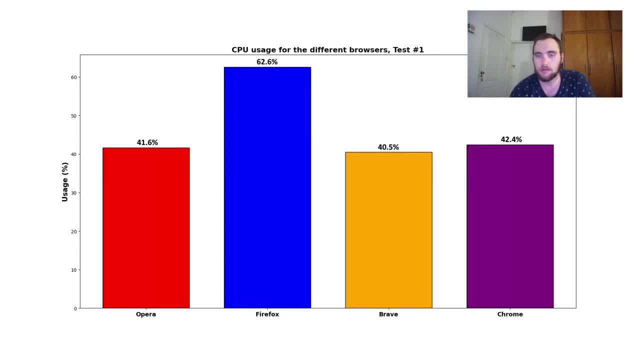 watching the video alone. you might be watching it and moving around, like looking at the comment section or maybe looking at a new video. you could be watching something. so i want to look at the worst case scenario and so you can see, in this worst case scenario, this simple test. 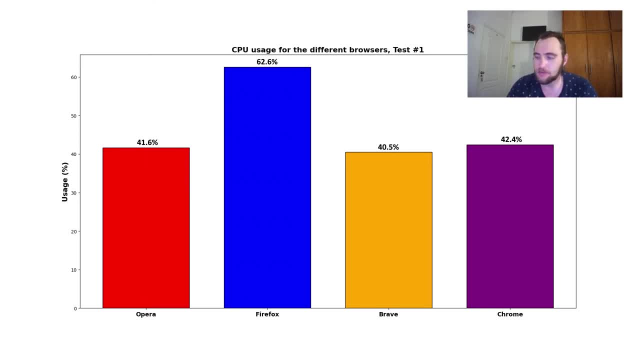 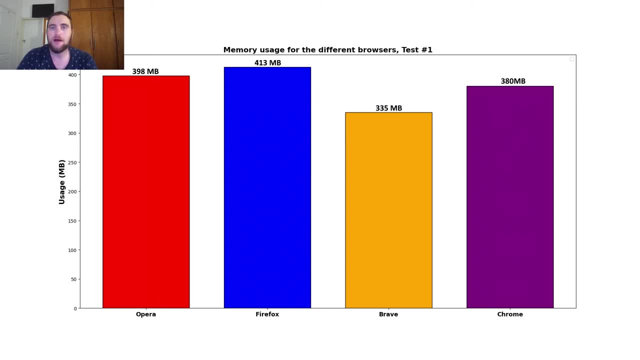 the brave browser did the best and mozilla firefox the worst. in terms of the memory usage, the brave browser did the best using the least amount of memory- 335 megabytes- with mozilla firefox using the most resources, at 413 megabytes at its worst. but the picture is different when we 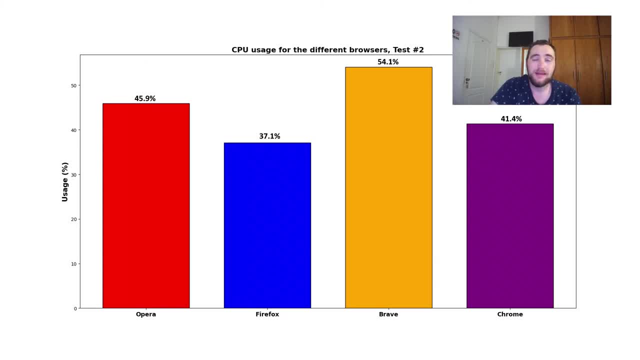 look at the cpu usage for test number two. when we have multiple tabs open now, the brave browser is doing the worst using at where? at this worst, 54.1 percent of the cpu, and mozilla firefox on the is using least at 37.1 percent. so let's be honest: in most cases you're not going to be using the. 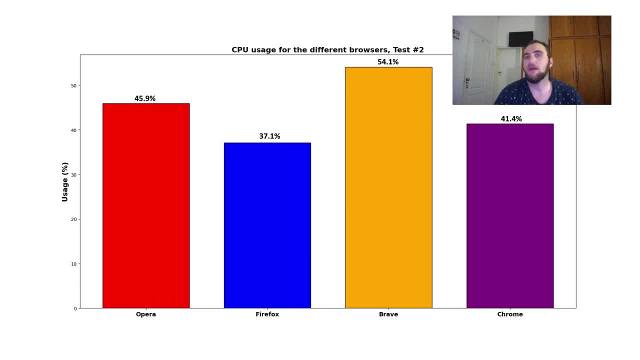 browser just for one tablet at a time. so in this case, just in terms of cpu usage, it seems like if you're going to be using multiple tabs or having multiple applications running in the background, mozilla firefox will be better in terms of the cpu usage. now, if we turn our attention to the memory usage, mozilla firefox is still the worst. 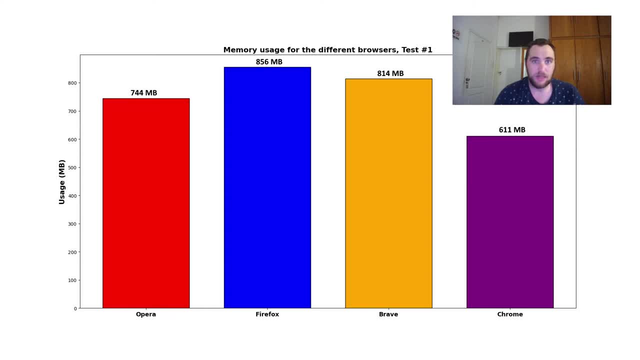 at 850 megabytes and mozilla firefox is still the worst at 856 megabytes. and, really surprisingly to me, google chrome did the best at 611 megabytes. i was so surprised at this result. i re-ran the test again for google chrome and i got 611 megabytes again. so i was really surprised with that one, because 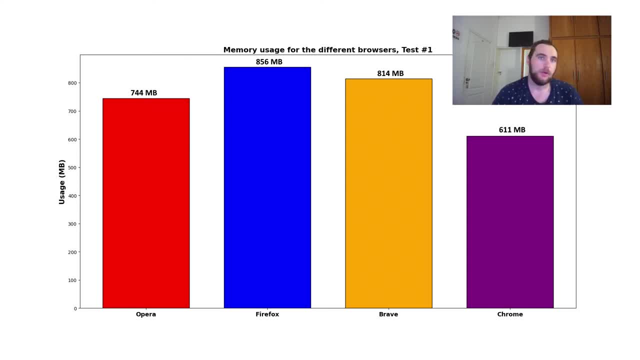 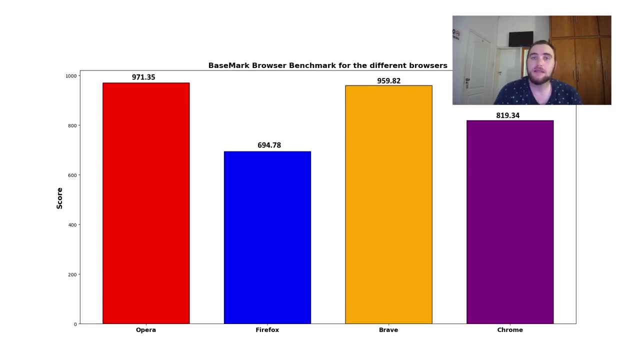 i actually uninstalled google chrome in the past because of the high memory usage and, um yeah, so that was a really good and surprising result for me. and the last set of results i want to look at is the basemark browser benchmark for these four different browsers. now, the higher the score is, the better the web browser is performing. 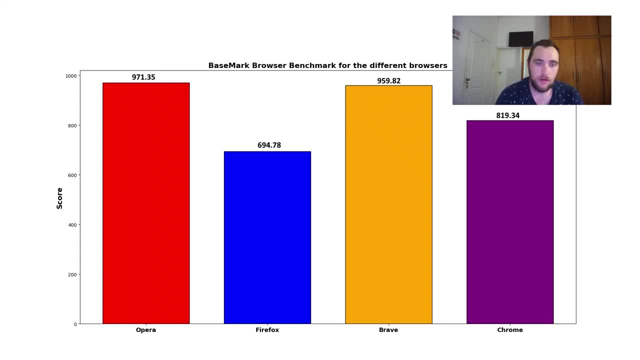 in this case, firefox has the lowest score and the high score goes to opera. so what this benchmark does is that it checks various different things. it's not just looking at the cpu usage, memory usage- it doesn't do that for so manyЬ. It looks at just how the browser is performing in terms of loading images, dealing with SFG files and a whole bunch of other things that I don't want to go over here. 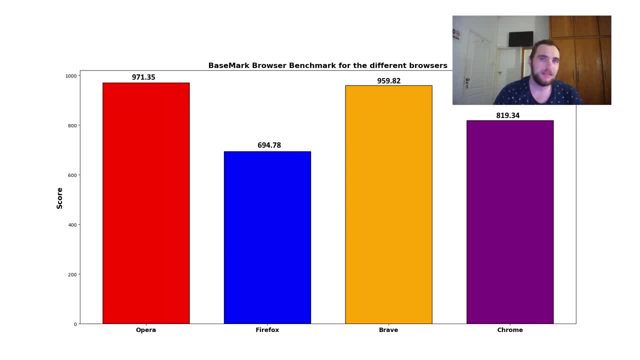 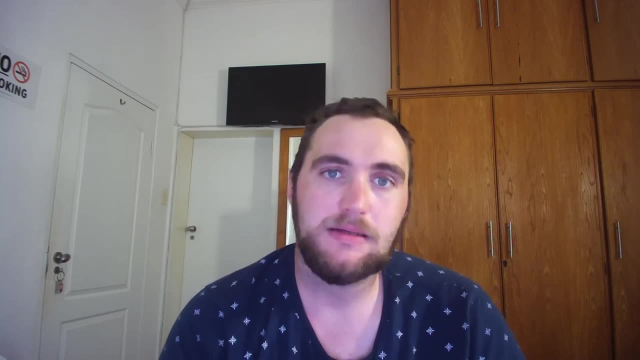 So, overall, based on the capabilities of the browser, the Opera browser is the better browser, followed by the Brave browser, and Mozilla Firefox is the worst. So, overall, in terms of just doing one thing at a time, the Brave browser is the best in terms of CPU and memory usage, based on this small set of tests. 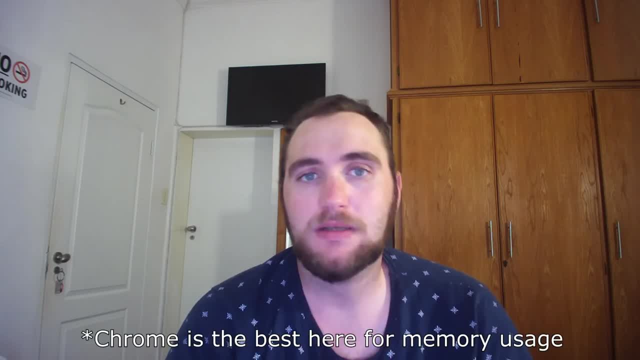 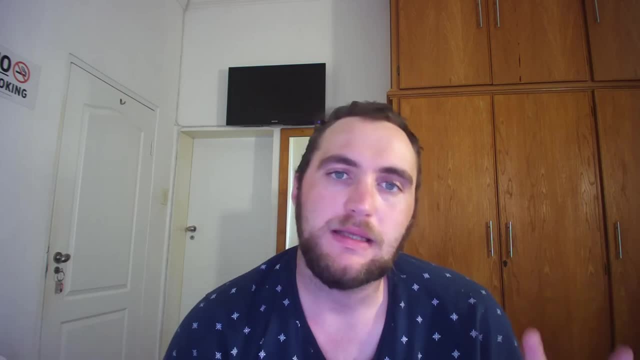 And if you're going to be doing multiple things at a time, Mozilla Firefox is the best for simple tasks, But if you want the browser that can do the most amount of things and do well at that performance, you can either try Opera or Brave browser.